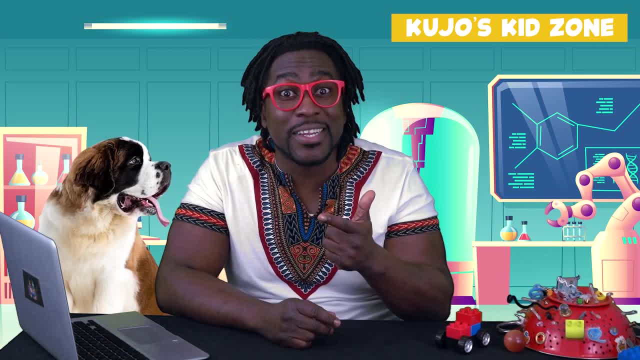 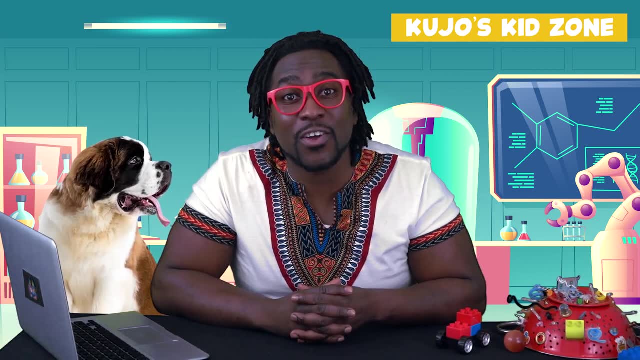 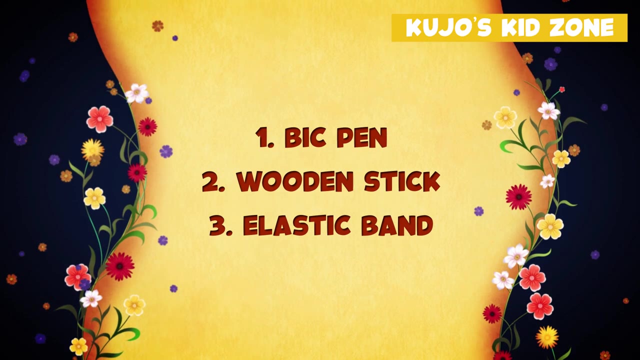 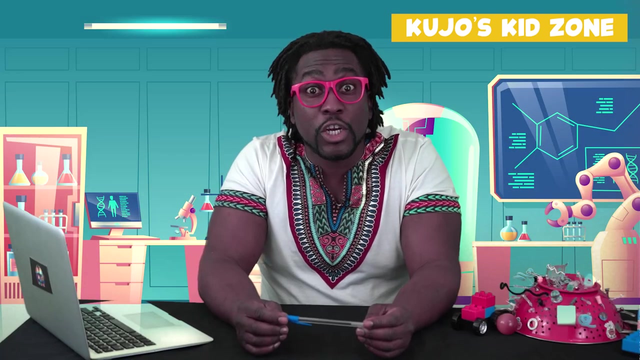 One A big pen, Two A wooden stick And three An elastic band. And we always have to remember to always ask a grown-up to help us. Okay friends, Okay friends, We're gonna show you a magic trick that will make you feel like you're in a good place. 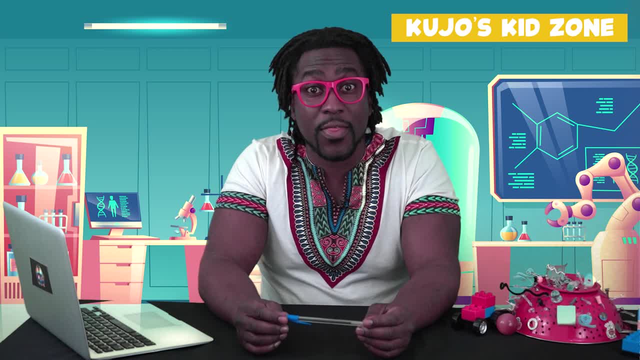 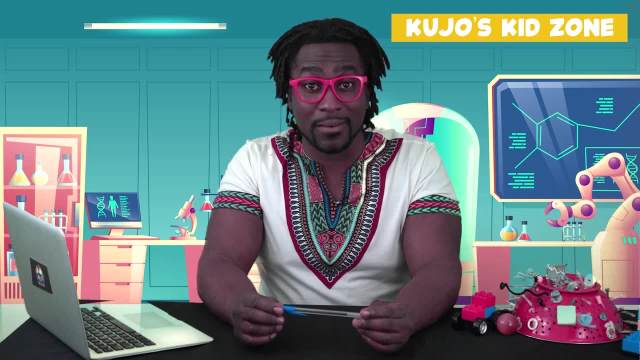 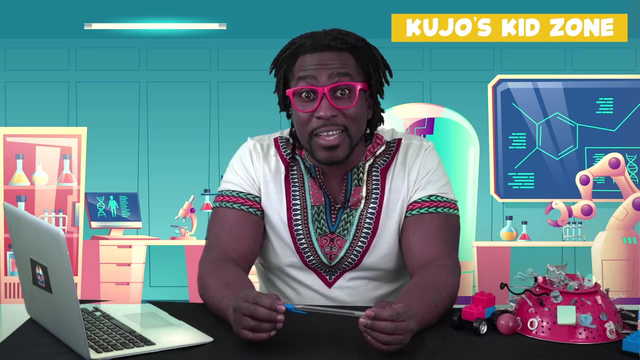 show you the first magic trick, and that's with a pen and a pen cap. It's very, extremely important that you use a big pen, because it's just much easier to do with this particular pen cap. So we're going to make this pen cap float onto this pen Watch. 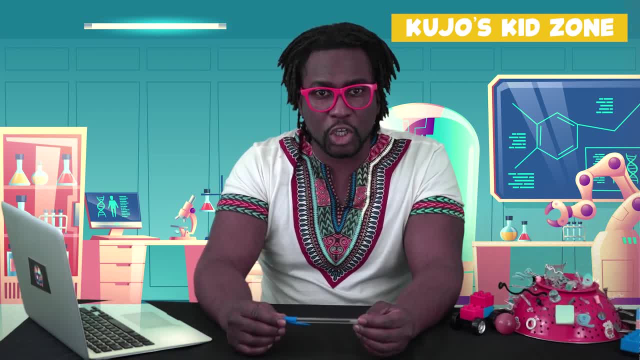 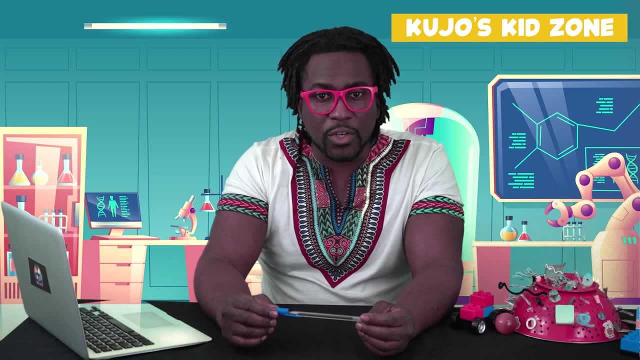 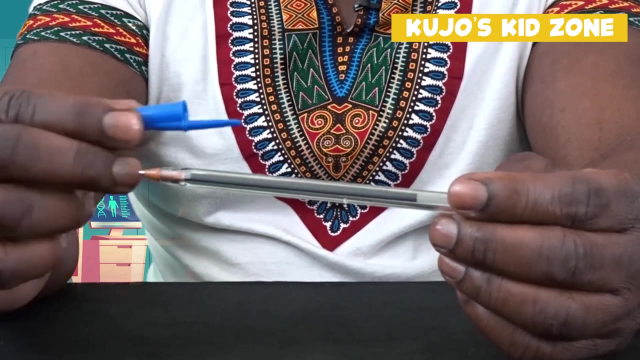 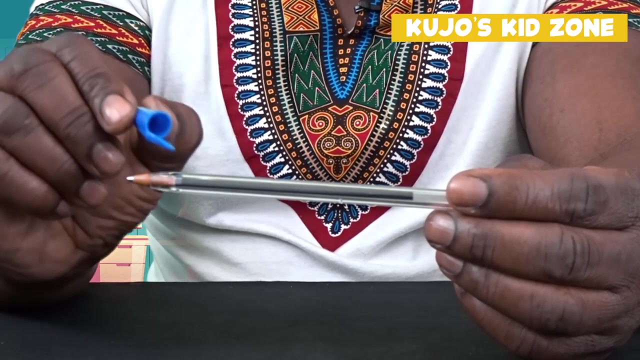 Okay, friends, woof. That happened super fast. Now let's go ahead and slow it down for you. Alright, step number one: We took the pen cap off, then we rotated it around: One, two, three. Then we come from the side: One, two and three. 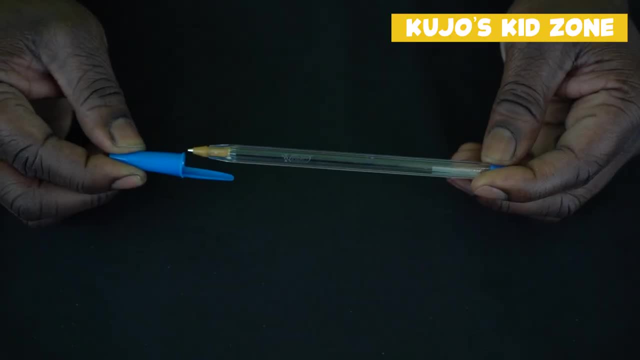 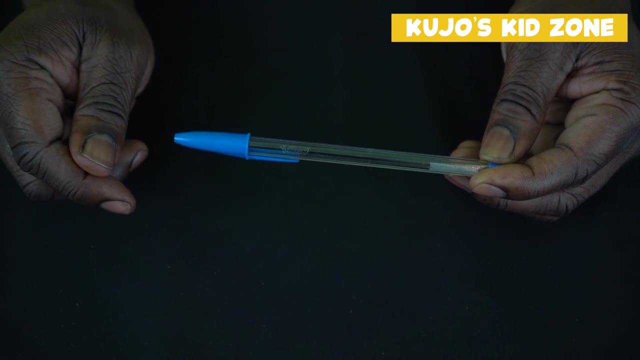 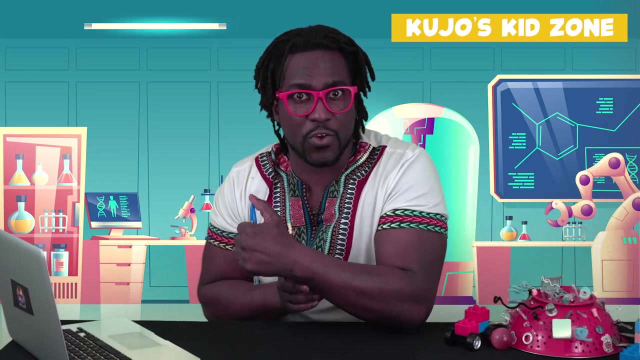 Then we bring the cap right back to the tip of the pen And we squeeze as hard as we can with our fingertips And voila, You have yourself a magic trick, And I'm going to show you now another magic trick that you can do. okay, 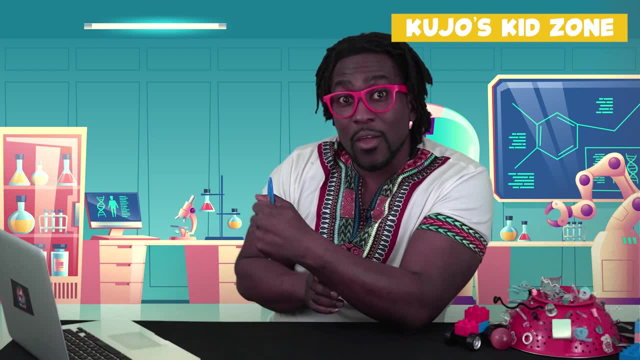 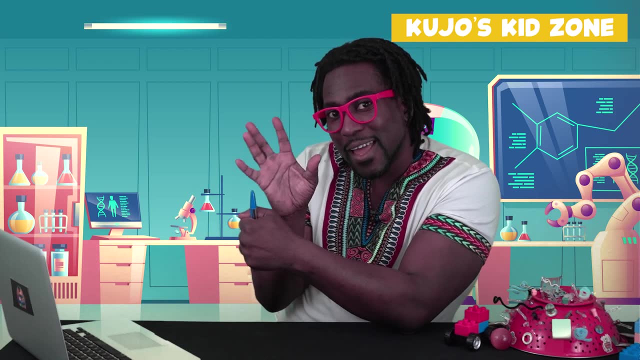 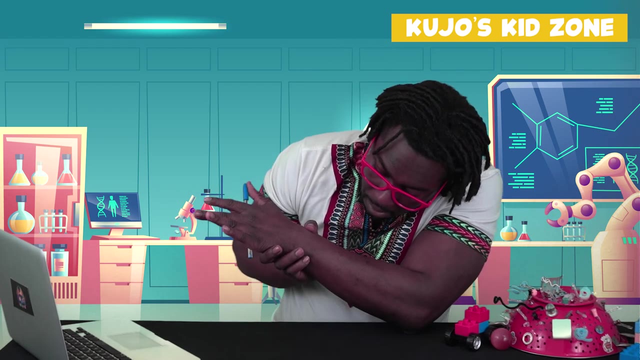 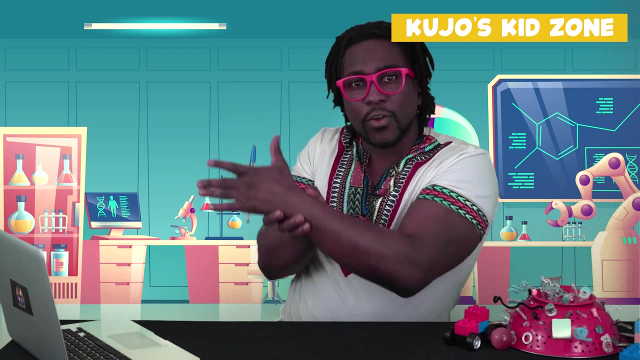 Using a pen as well, The same pen. We're going to make it float. So you got to take your pen and put it in your hand like this: Oh wow, Oh wow, Oh wow, It's floating. You have a floating pen. 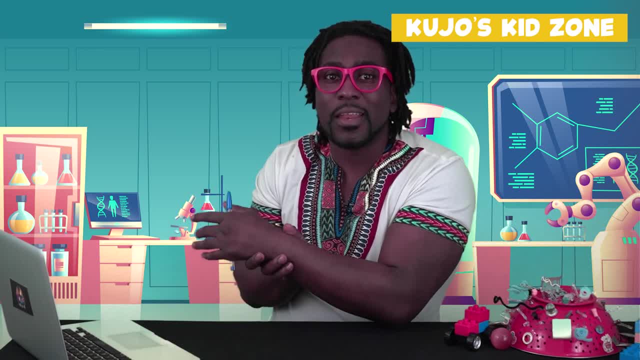 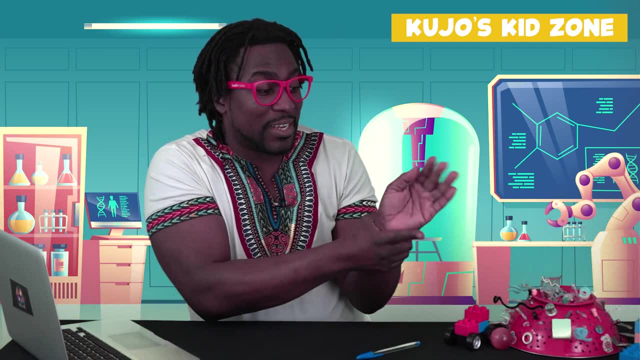 Okay, how does it really work? Now? this is what it looks like on the other side. So you're holding your wrist, You're holding your wrist like this And you have one finger, your index finger, that's holding the pen. 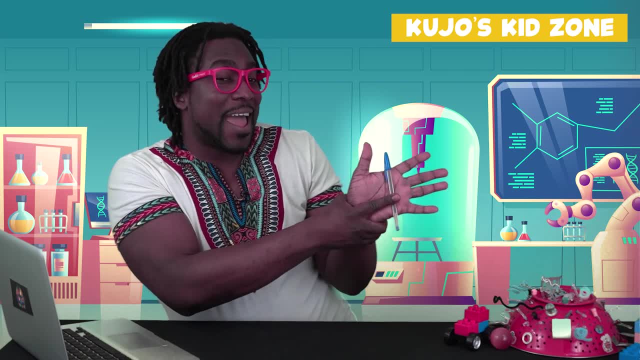 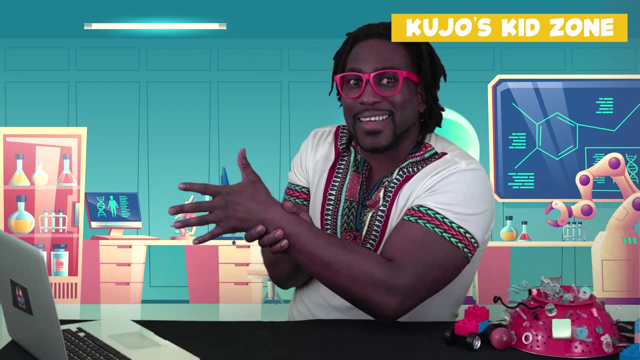 So it's like this: You're holding the pen like that, but this is how it looks like on your side, But when you show it to your friends and your family, it's going to look like this. So it gives the illusion that it's floating, when it's really not. 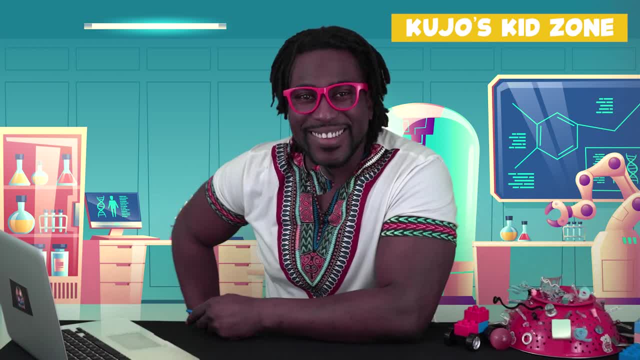 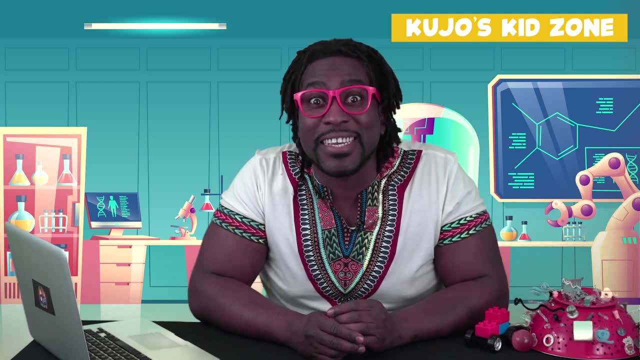 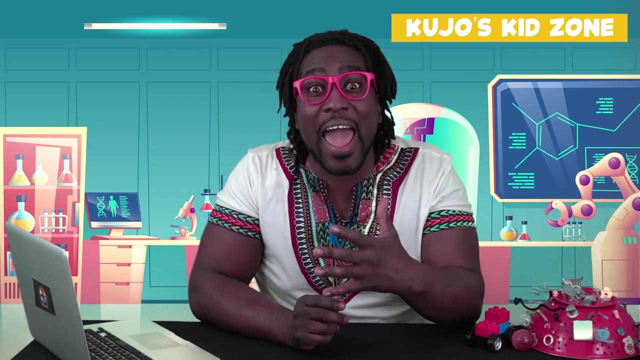 And that's what magic is all about. Now that we've done our first magic trick, let's focus on doing a second magic trick. I know one that's more cool even than the first one. We're going to make the same pen float by using our hands. 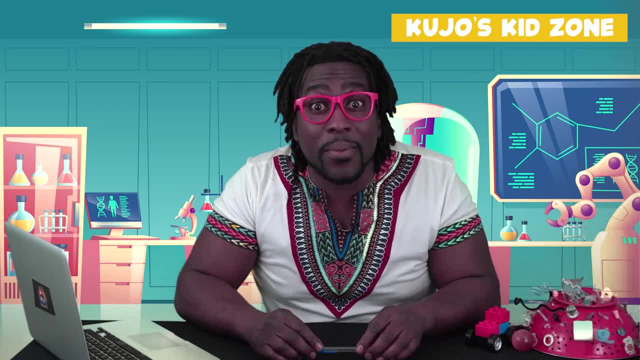 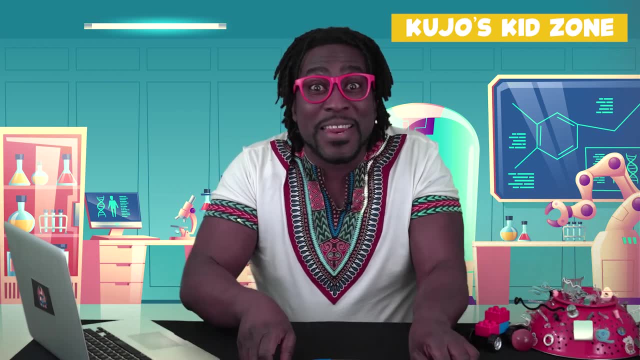 I'm going to show you how to do that. So we need to have a couple of things: One, the exact same pen. We need a wooden stick, We need an elastic band And, oh yeah, we should probably get a mirror. 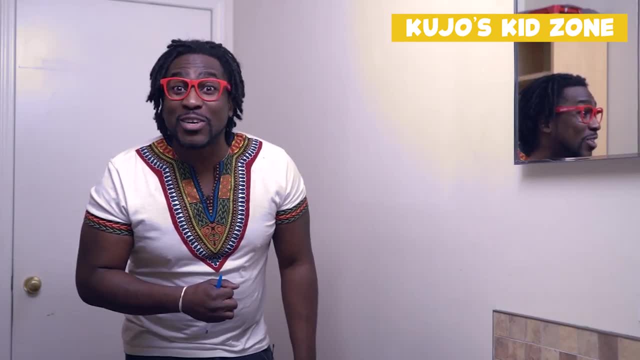 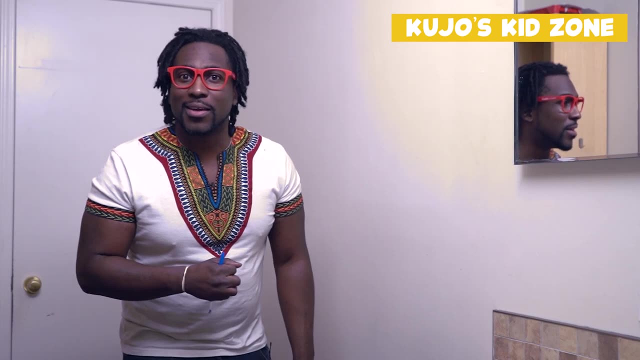 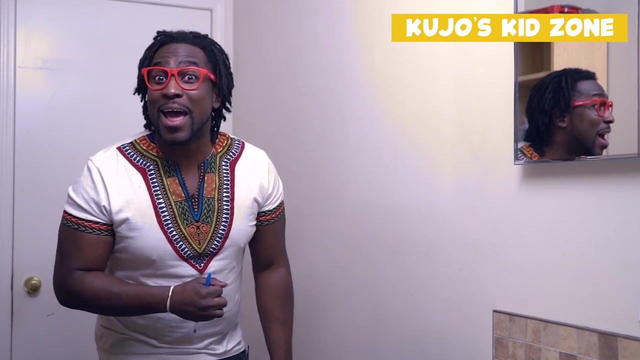 Alright, now that we've done the first magic trick using the pen, I'm going to show you another cool magic trick. Watch this: We're going to make the pen float. Last time we made the pen cap float. Now we're going to make the whole pen float. 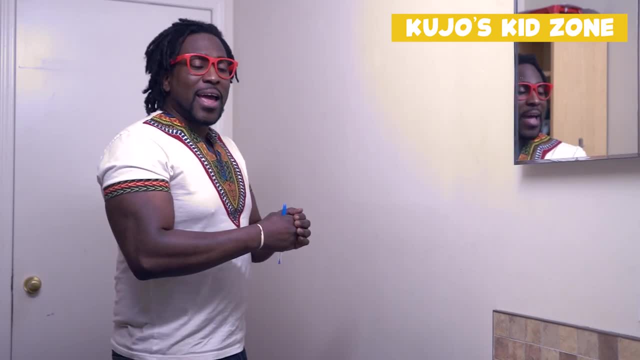 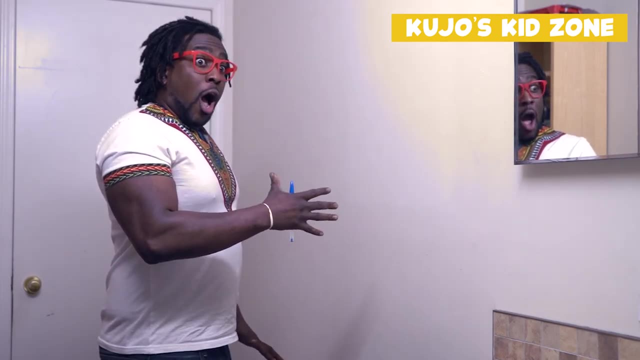 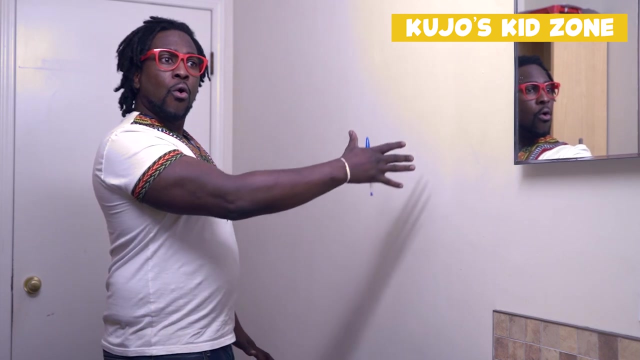 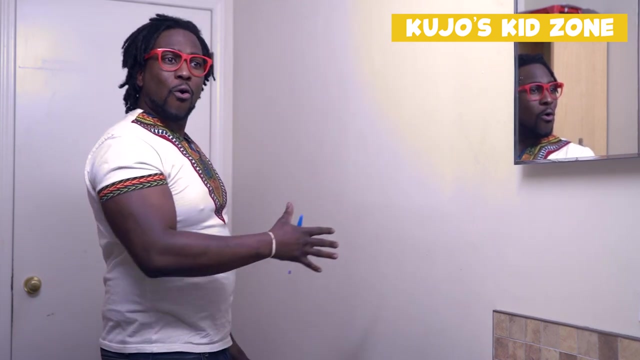 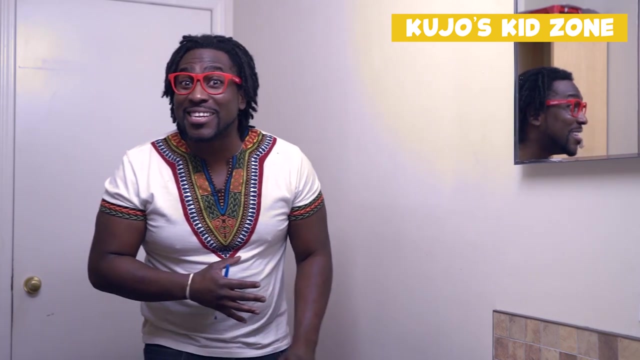 Watch this. Close your hand I'm squeezing. Oh cool, eh. Now I'm going to show you how it works. What you don't know and what you didn't see is this: I have an elastic band. Remember, I told you about that wooden stick. 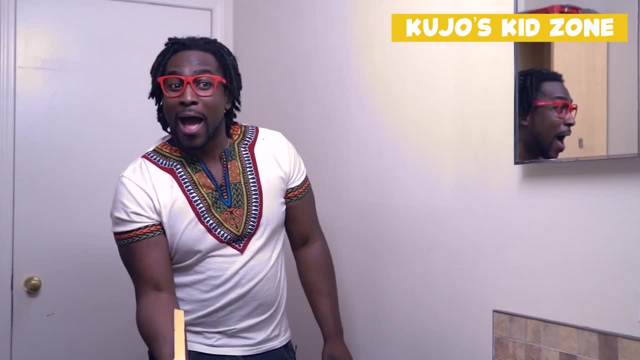 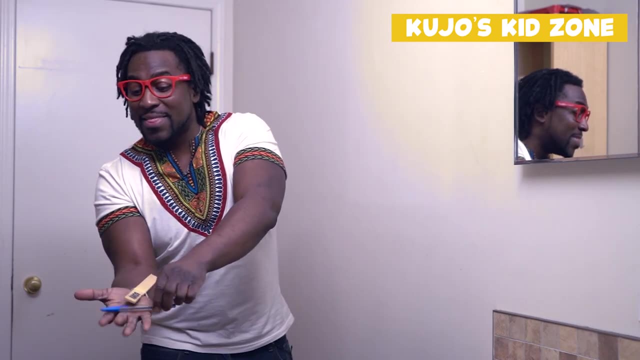 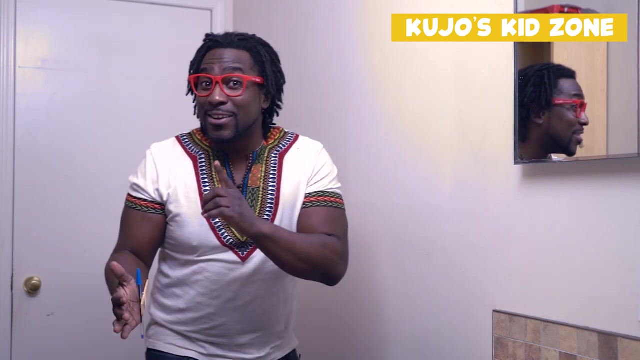 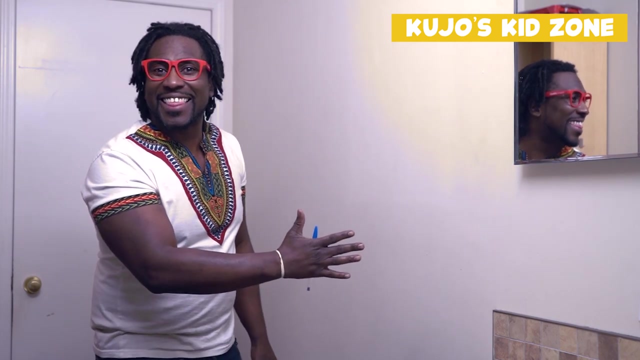 Watch this. You see the wooden stick And the elastic band is holding it, And then the pen is being held by the wooden stick, You see, But when we show it from a certain angle, you can't see nothing. You won't see nothing. 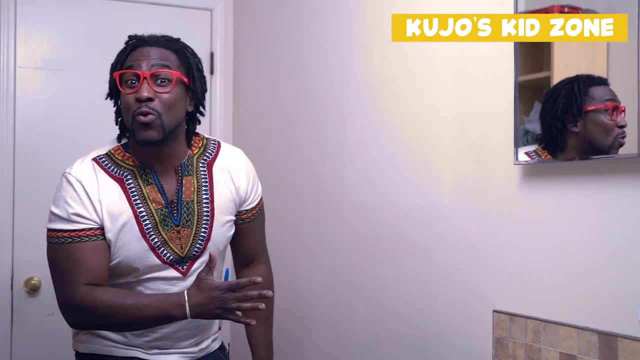 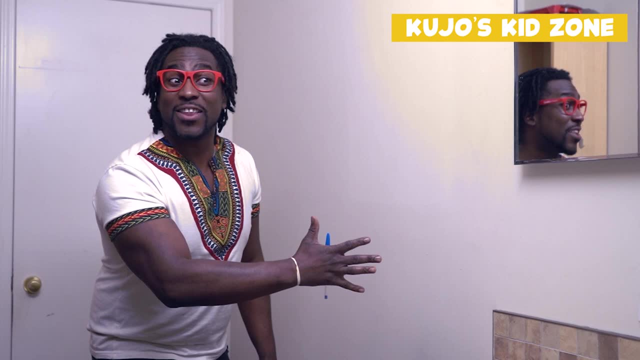 And neither will any of your friends or family. when you show them the cool magic trick, Watch this. You start off, you're holding it And then you extend your hand and woof, woof. Look at that angle. They won't see anything. 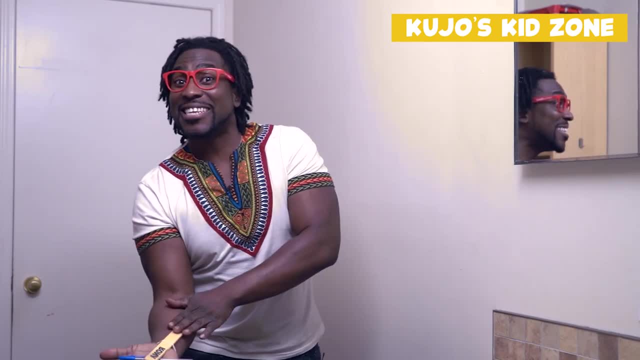 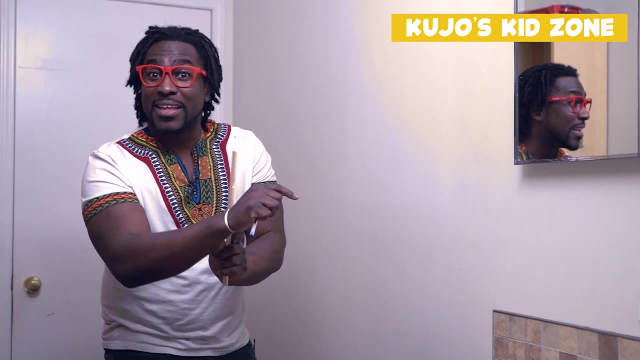 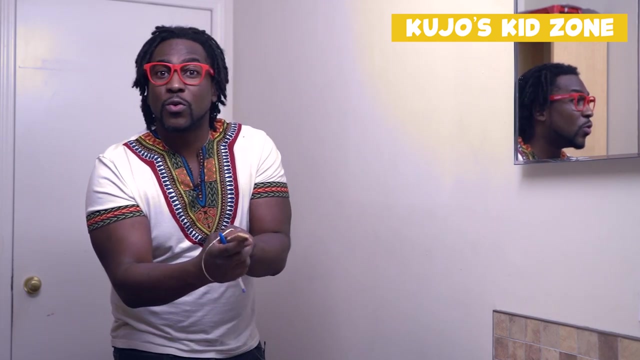 But you and I know that you got a wooden stick that's holding your pen. Now you try it. You take the elastic, You put in the wooden stick, Or you can even use one of those ones that you eat for sushi- A chopstick. 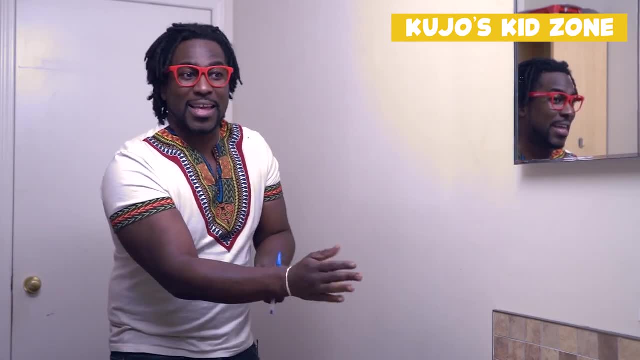 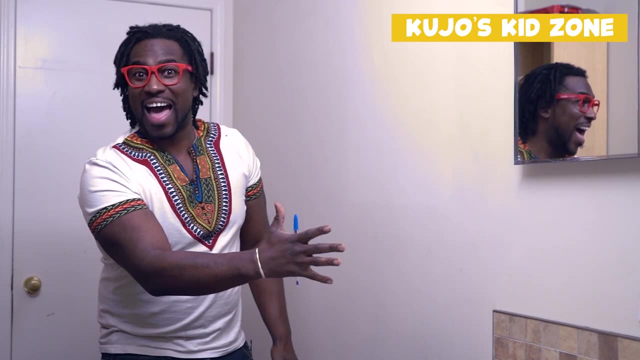 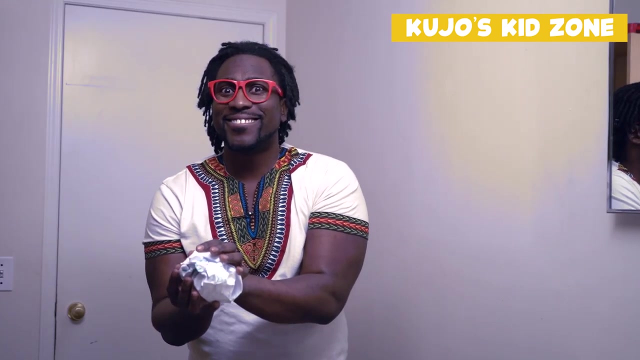 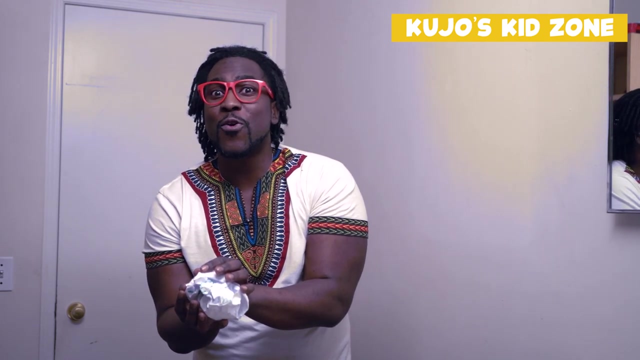 You hide it behind your hand like this, And then you put your pen right inside And look, Voila, Magic. Alright, everyone, I have shown you two magic tricks And I said I wouldn't do it, But I'm going to show you a third magic trick. 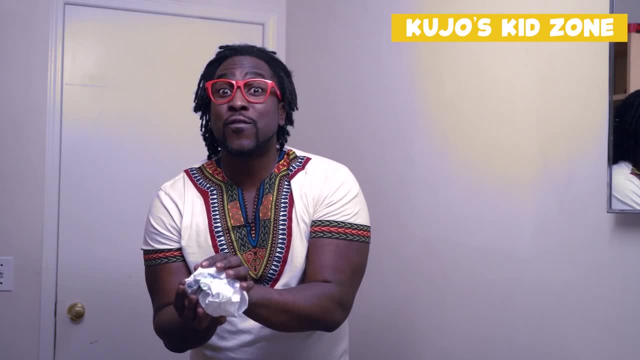 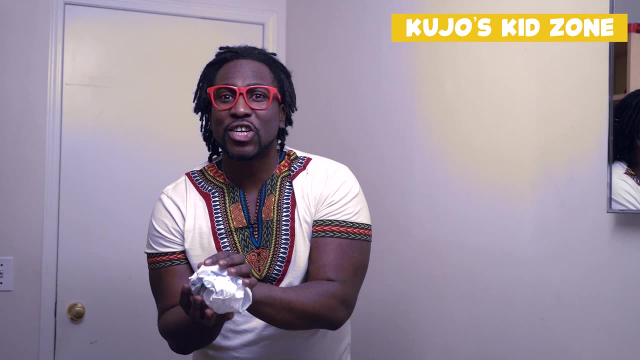 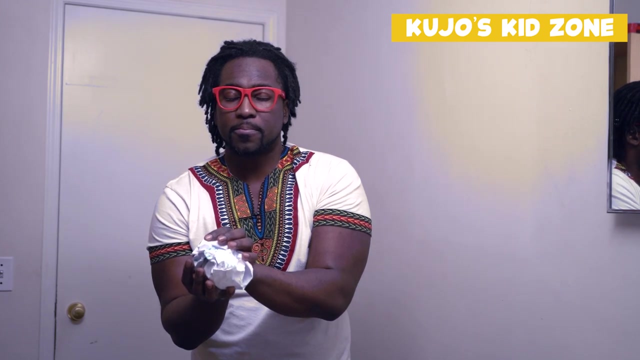 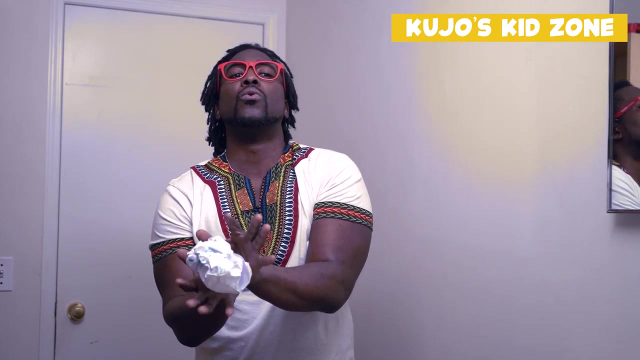 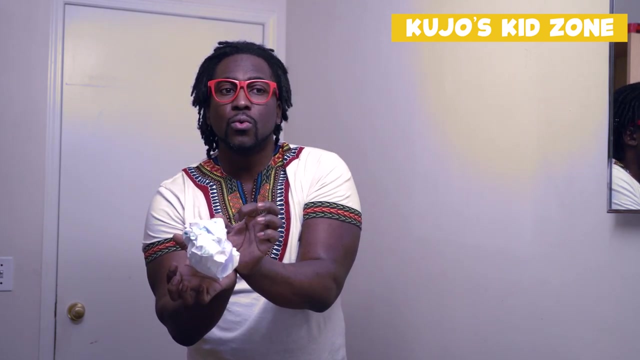 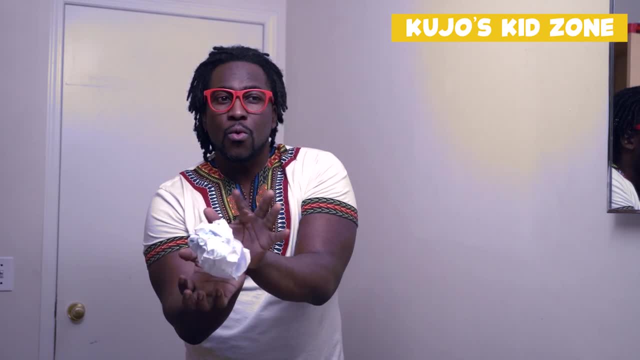 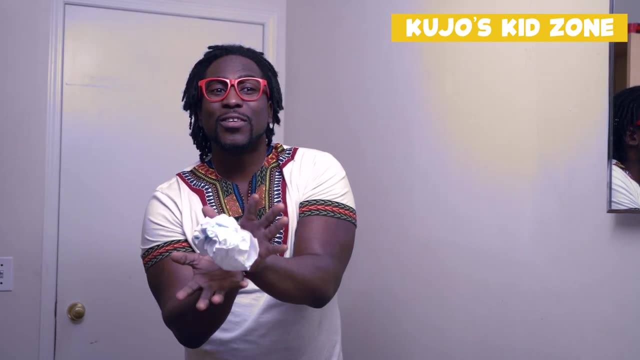 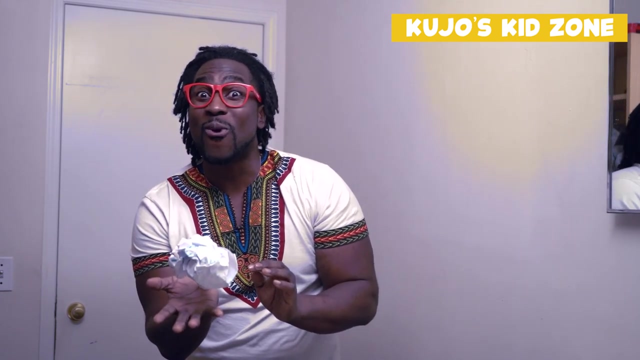 Woof, Woof, Woof, Woof, Woof. And here we go, It's floating. See how it's floating. Now I'm going to show you how it works. Watch this. So remember, we had the elastic band. 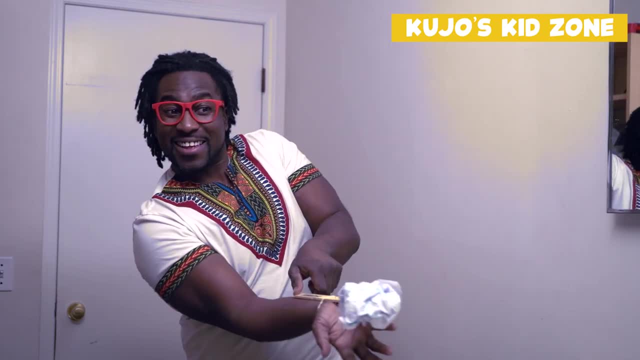 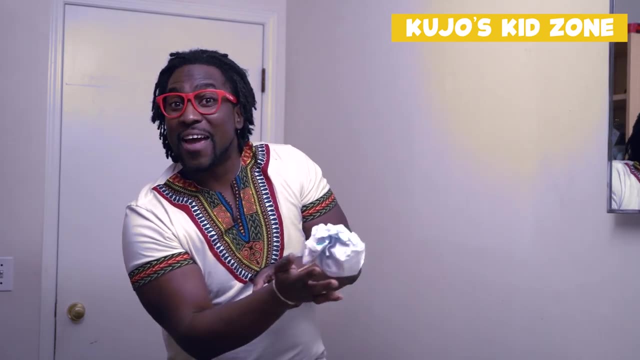 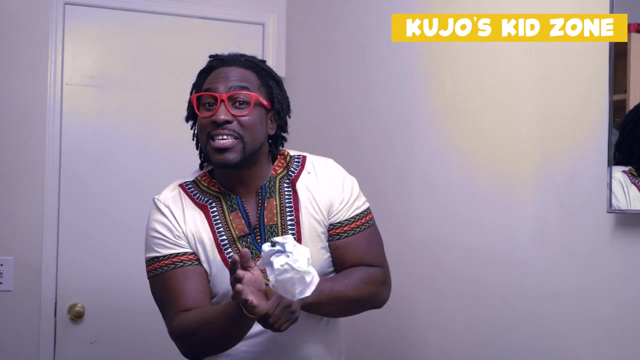 And remember, we had the wooden stick, we had the wooden stick. so we have the elastic band and we have the wooden stick. But everything is all about angles. So if we show you from a different kind of a view, you won't see the wooden stick. 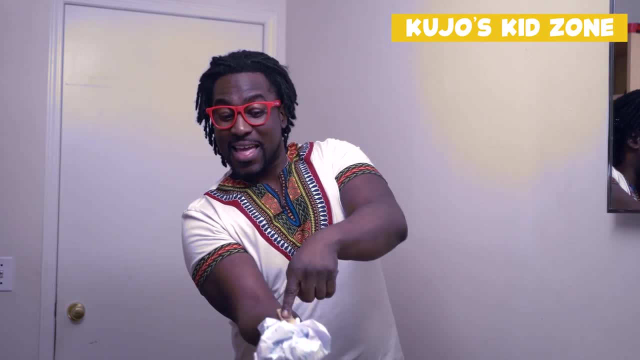 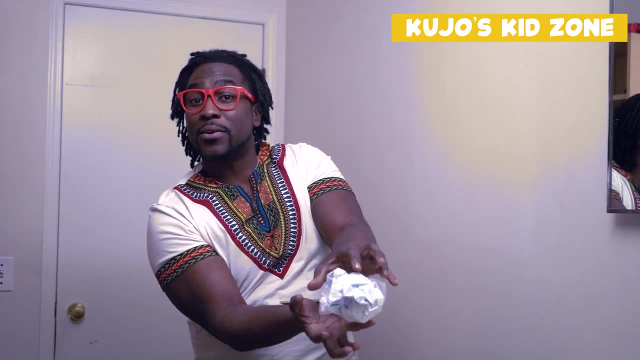 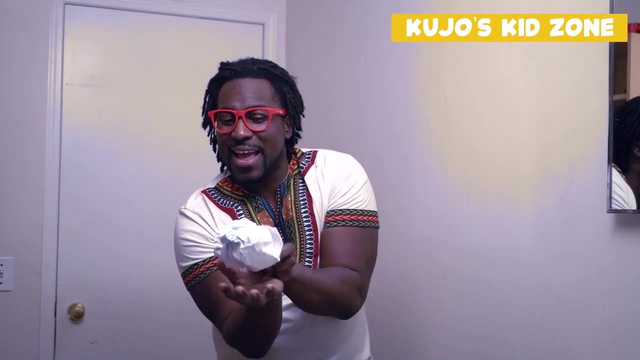 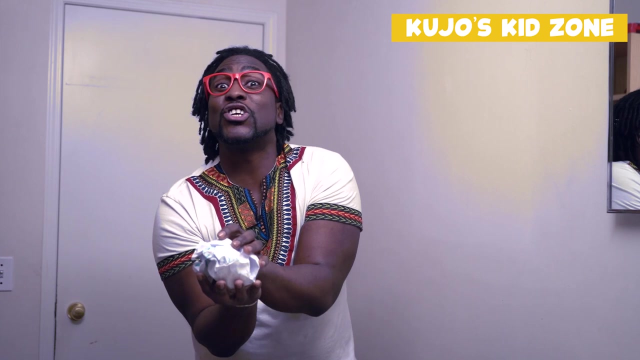 So you take the wooden stick the same way, the same way, and you put it right here where your wrist is. You take a piece of paper that you were going to recycle anyway and you attach it to the wooden stick. But when you show from this angle, you crunch the paper and then you dig deep in yourself as a distraction to show the ball floating. 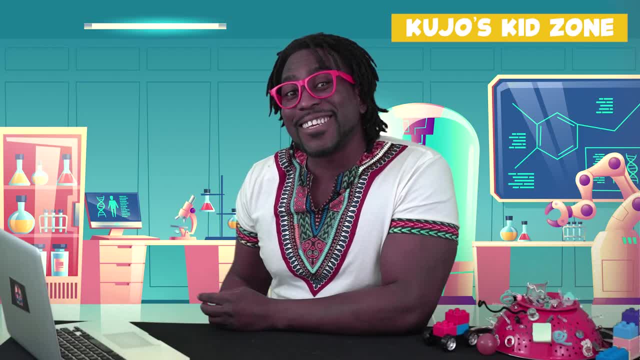 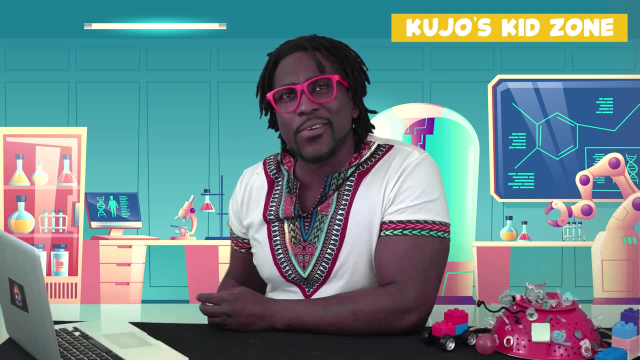 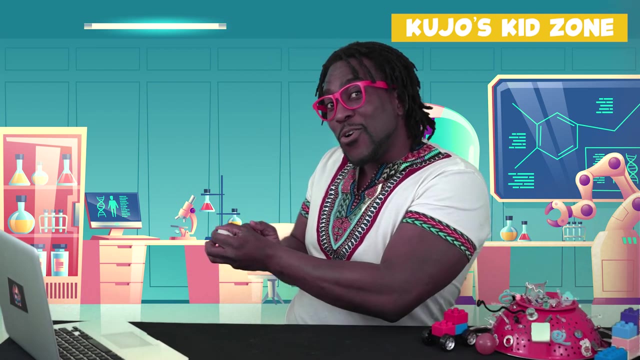 Magic. Hey, Michaela, I wanted to give you a special thank you for asking me To show you one of my most favorite things in the world, which is to do magic tricks. So thank you. thank you so much for asking me to show you how to do some magic.